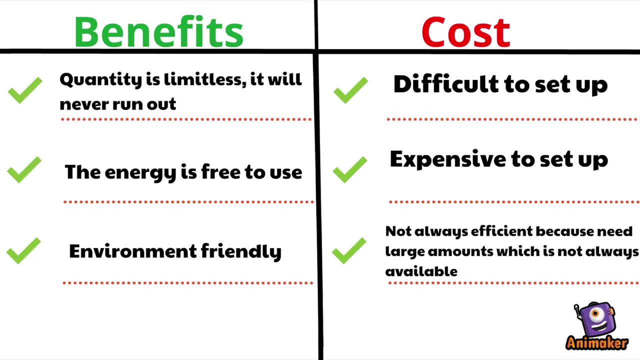 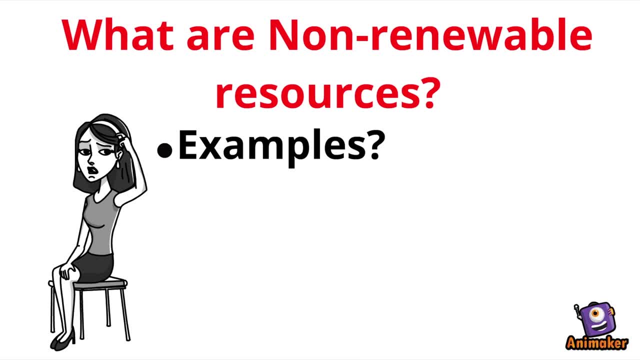 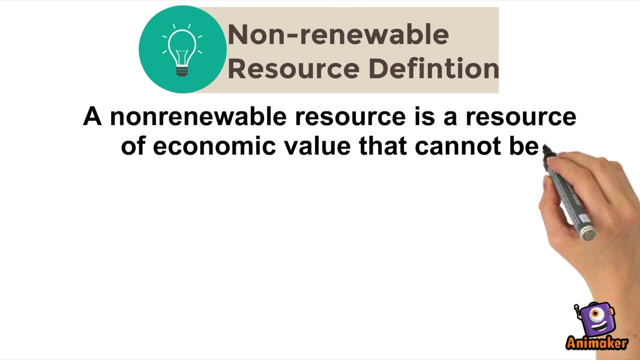 always efficient because we need large amounts, which is not always available. So, now that you know this, what are non-renewable resources? Examples: Costs, Benefits. So what a non-renewable resource is? It's just basically a resource of economic value. 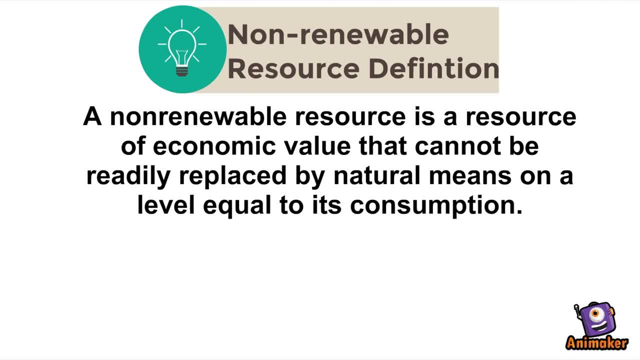 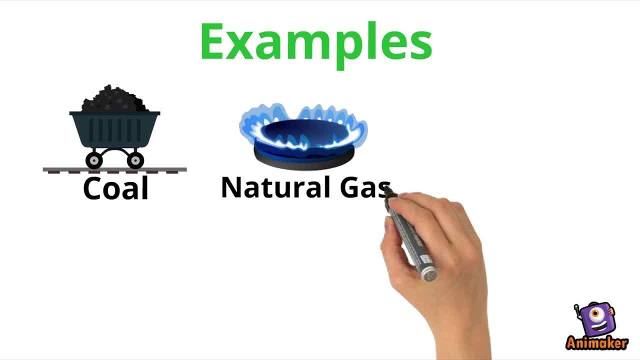 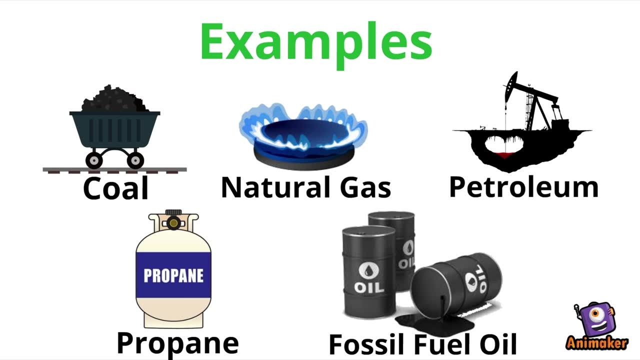 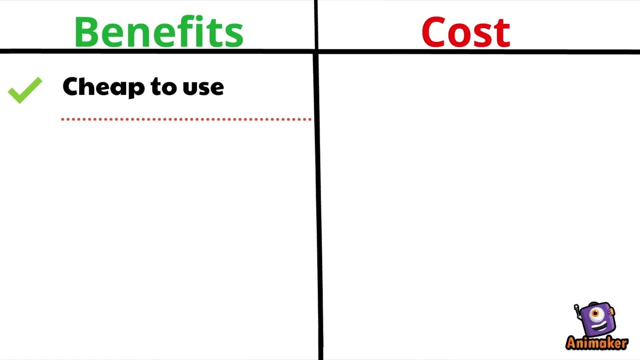 that cannot be readily replaced by natural means on a level of equal to its consumption. Some examples are coal, natural gases, petroleum, propane and fossil fuel oils. The cost of benefits of non-renewable resources are: it's cheap to use, it's easy to use, it's efficient and it only requires a small amount to. 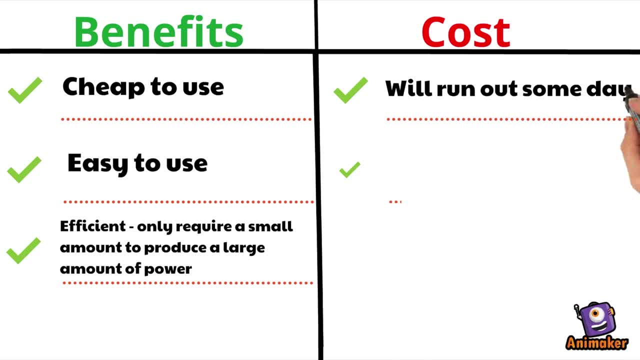 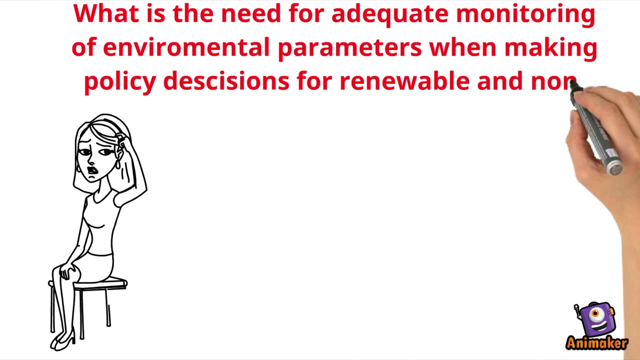 produce a large amount of power, The costs are it will run out someday, causing serious environmental changes, and it releases toxic gases which are contributing to global warming. What is the need for adequate monitoring of environmental parameters when making policy decisions of renewable and non-renewable resources? Well, that's a. 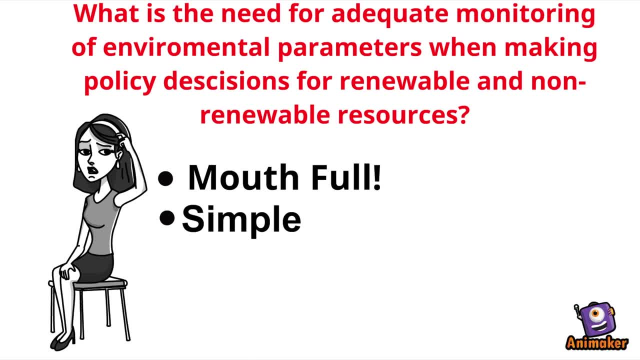 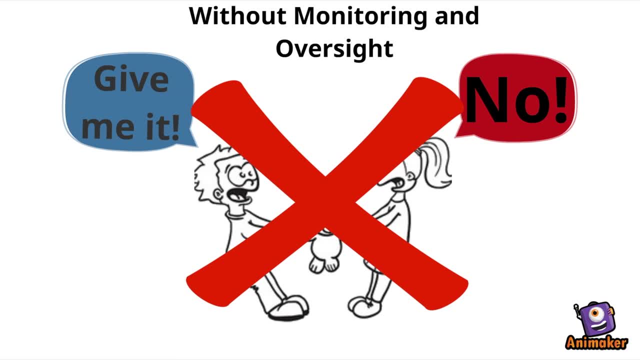 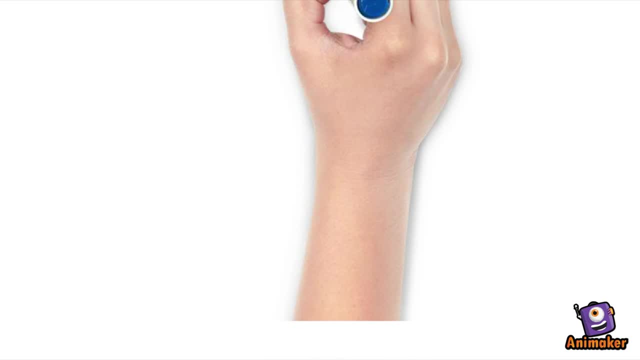 mouthful. Let's make this simpler by showing an example. So imagine two kids in a playground fighting with a teddy bear, with no monitoring and oversight. well, that's not good, because one kid will get hurt, and we don't want one kid to get hurt because that's pretty sad. so with the 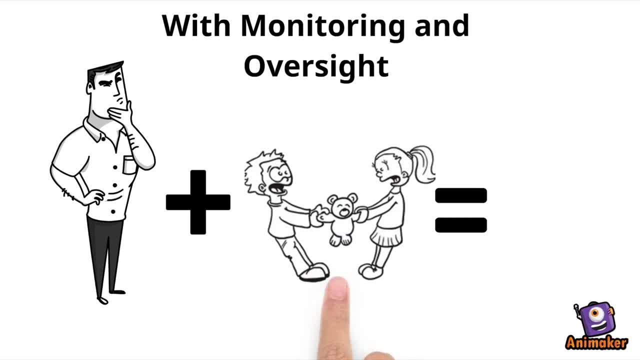 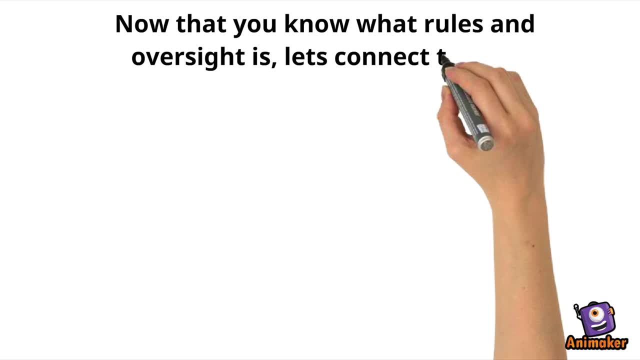 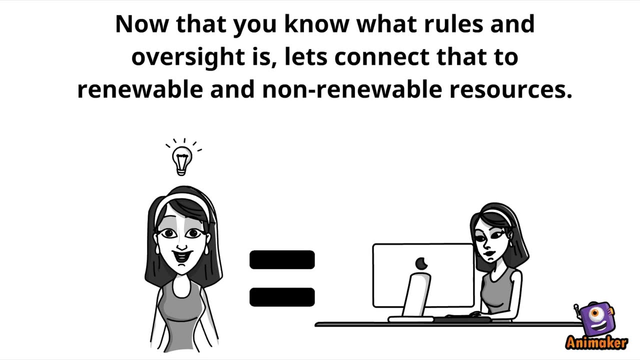 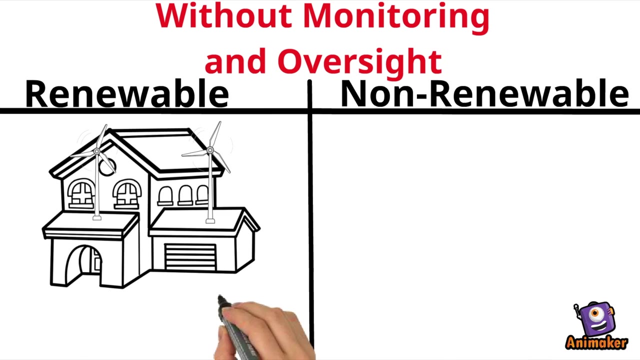 teacher representing the government, as the ones monitoring and overseeing the children while they're playing. results and happy children. now that you know what rules and oversight is, let's connect that to renewable and non renewable resources, because that's a good idea. so, without monitoring and oversight with renewable and non renewable resources is with renewable. 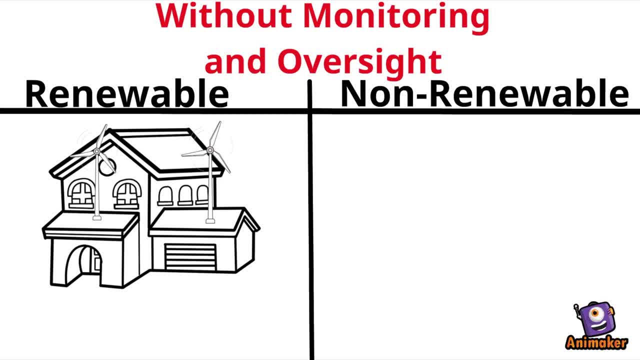 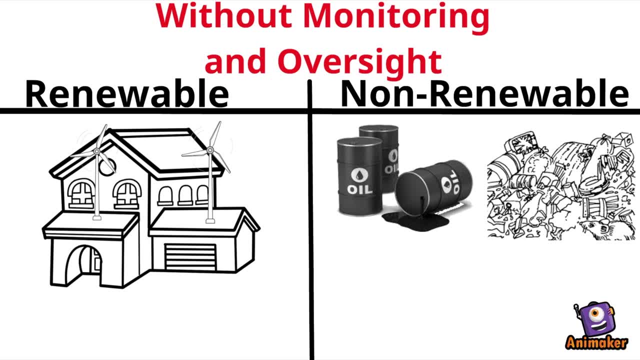 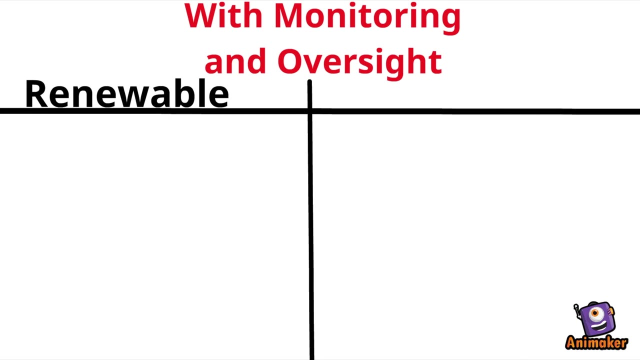 just imagine you have a house and windmills on top. that's pretty messed up and there'll be unnecessary oil spills and unnecessary and large amounts of pollution. that would be crazy. one meals on your house, am i right? haha, you get it so with monitoring and oversight, with renewable and non.